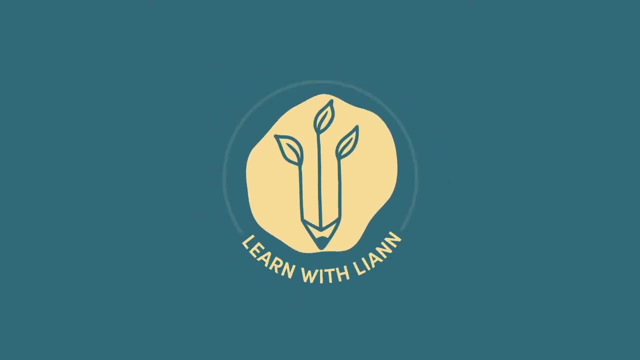 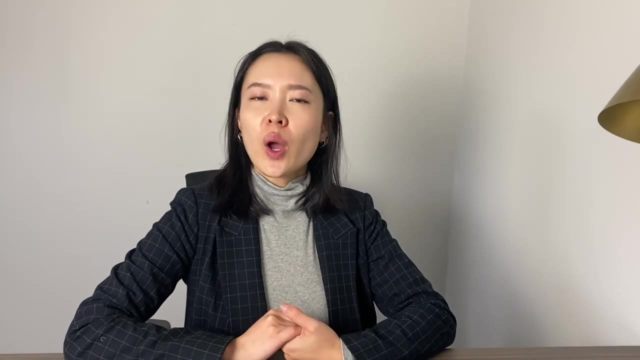 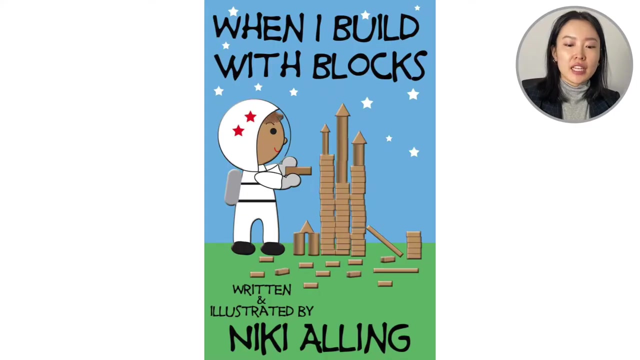 Hello everyone, welcome back to Reading with Lianne. Today we are going to read the book When I Build with Blocks. This is written and illustrated by Nikki Arling, So looking at the cover of the book, we see a boy building, building with blocks, building a castle or maybe a spaceship. 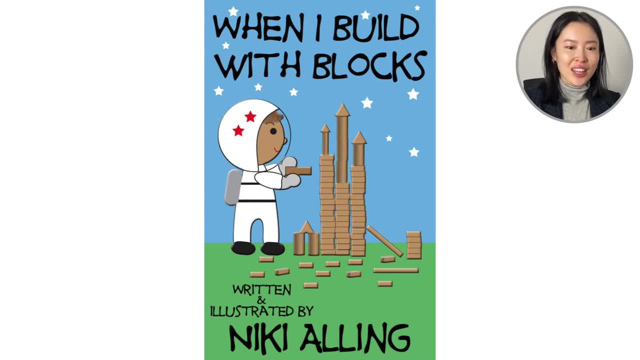 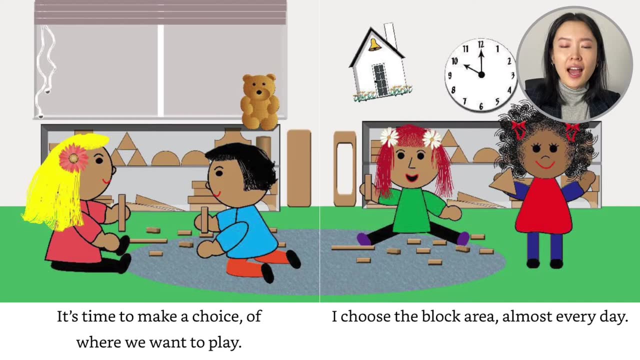 because he's an astronaut. Let's see all the things that we can build. It's time to make a choice of where we want to play. I choose the block area almost every day, So it looks like we're in the classroom. right There's shelves of blocks. Kids are learning about the time. 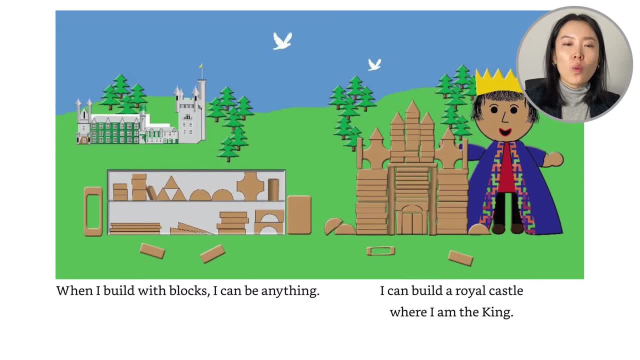 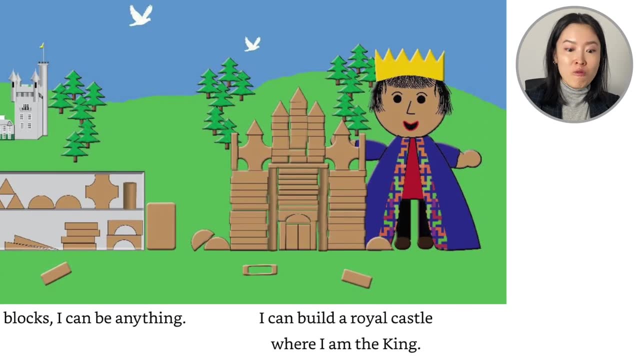 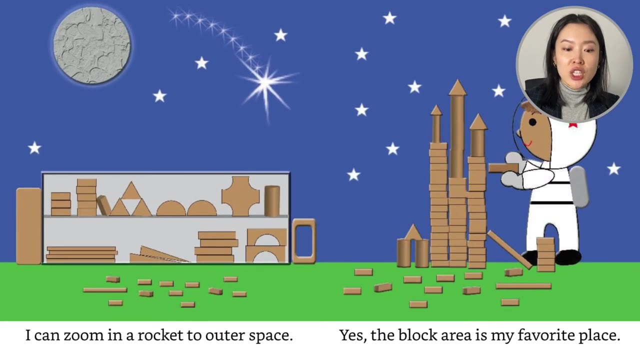 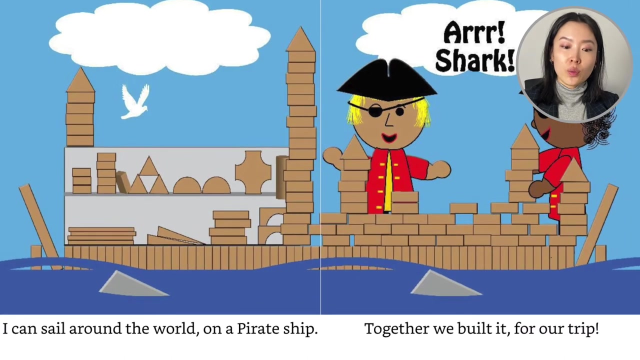 They're learning about ABCs. When I build with blocks, I can be anything. I can build a royal castle where I am the king. I can zoom in a rocket to outer space. Yes, the block area is my favorite place. I can sail around the world on a pirate ship. 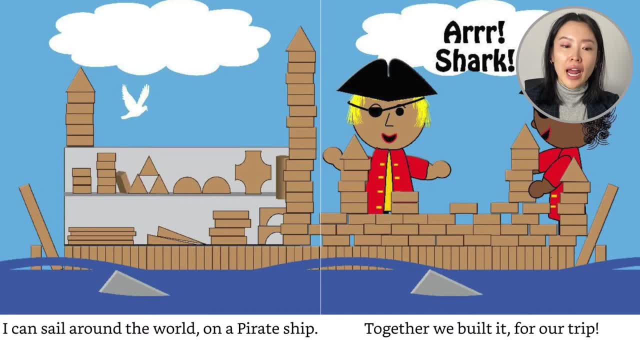 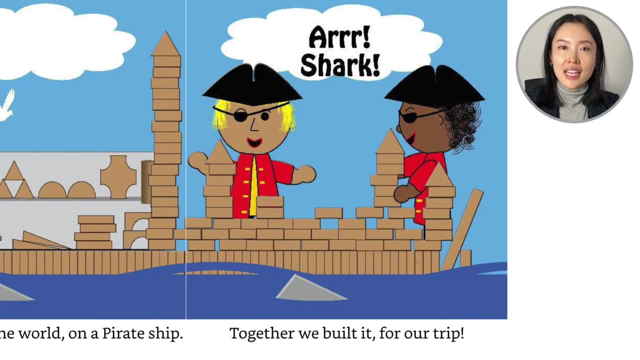 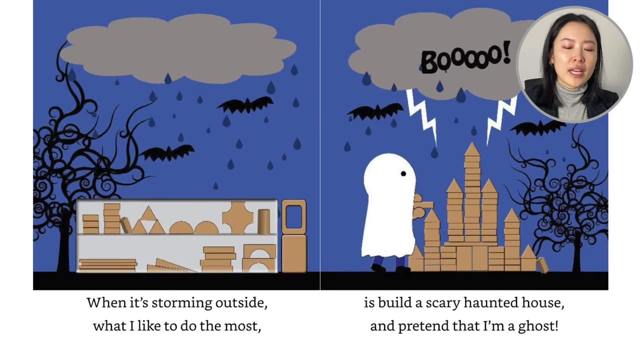 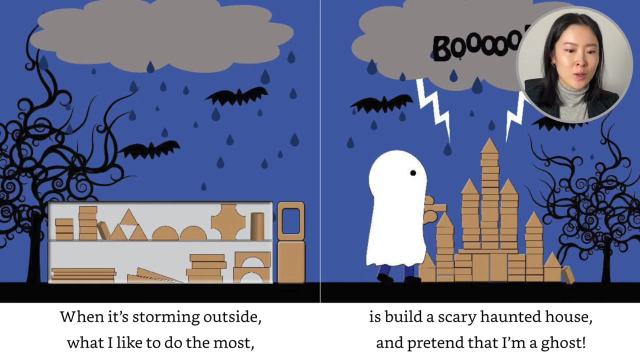 Together we build it for ourselves. trip. Look at their eye patches with their pirate hats. When it's storming outside, what I like to do the most is build a scary haunted house and pretend I'm a ghost. Look at the wacky trees, the storming clouds, the lightning, the bats. 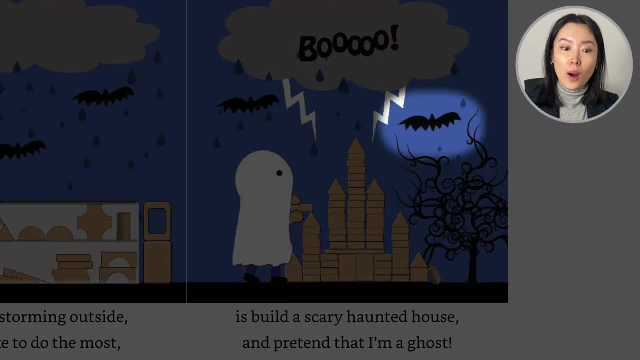 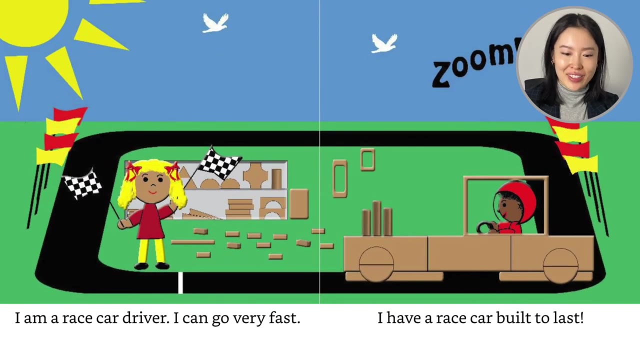 1,, 2,, 3,, 4,. Ooooo, I am a race car driver. I can go very fast. I have a race car built to last, So the girl she's at the starting mark and she waves the flag and the boy can zoom across the track. I am a firefighter.